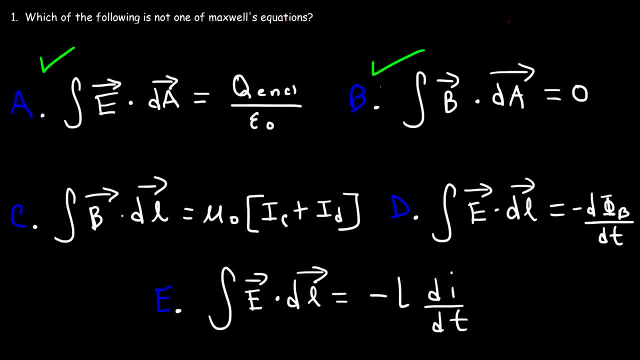 And that is Gauss's law for magnetic fields, Which states that the total magnetic flux through a closed surface is always zero. Now the third one is also one of Maxwell's four equations, And this is Ampere's law. This is the permeability of free space. 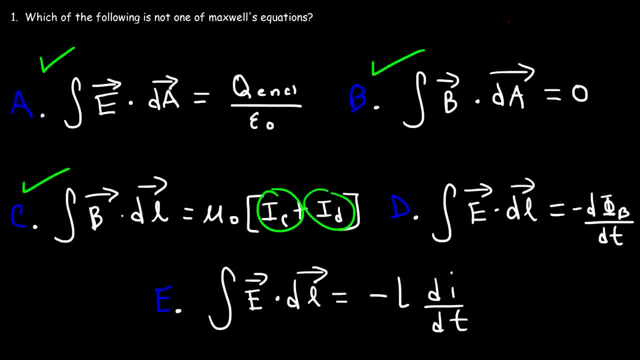 Ic is the conduction current, Id is the displacement current, So this entire expression represents the enclosed current Answer. choice D is also one of Maxwell's equations and it's associated with Faraday's law. A change in magnetic flux can induce an electric field. 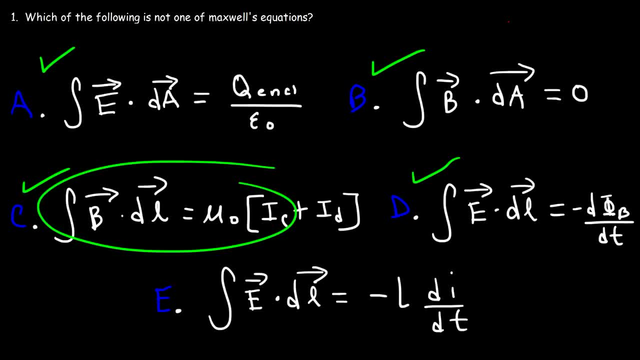 And for answer choice C, you need to understand that both the conduction current and the displacement current can act as sources of a magnetic field. And for E, this is just the EMF of an inductor And this is the EMF of an inductor. 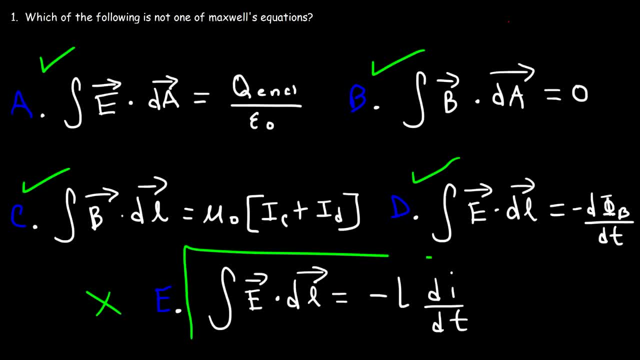 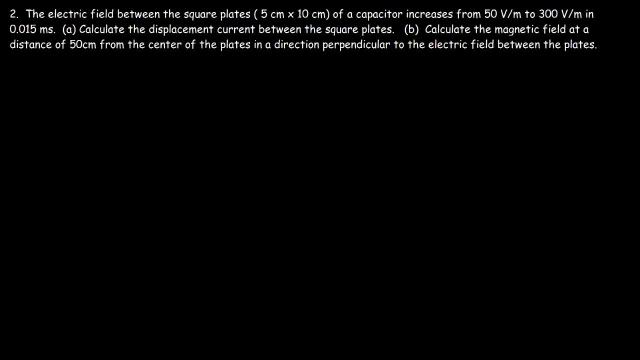 And this is just the EMF of an inductor, And this specific equation is not listed as one of the four of Maxwell's equations. Number two: The electric field between the square plates of a capacitor increases from 50 volts per meter to 300 volts per meter in 0.015 milliseconds. 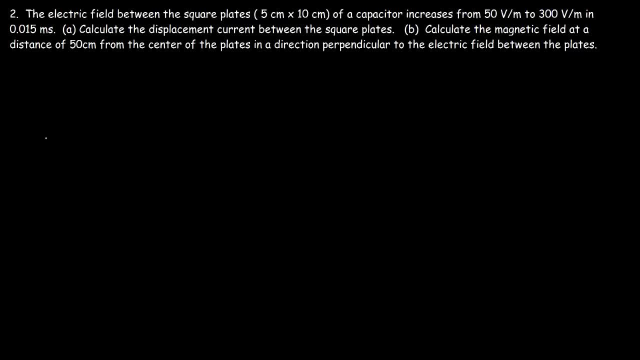 Calculate the displacement current between the square plates. So let's start with a picture. So let's say this is the side view of the plates of a capacitor And let's say this plate is positively charged and this plate is negatively charged, And so we have an electric field that emanates from the positive plate and is pointed towards the negative plate. 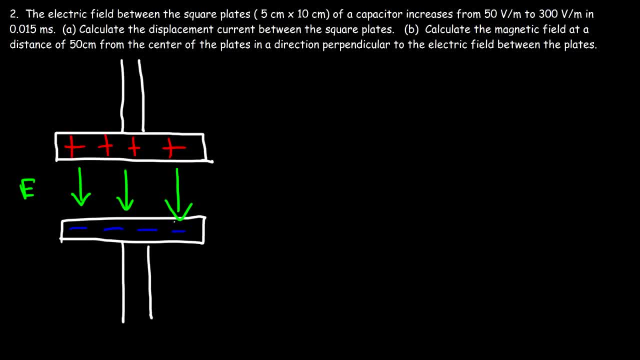 And let's say, the capacitor is charged up right now. So the current that flows in that section, that is the conduction current, Now the displacement current is technically a fictitious current, which is represented by the change in electric field in between the square plates. 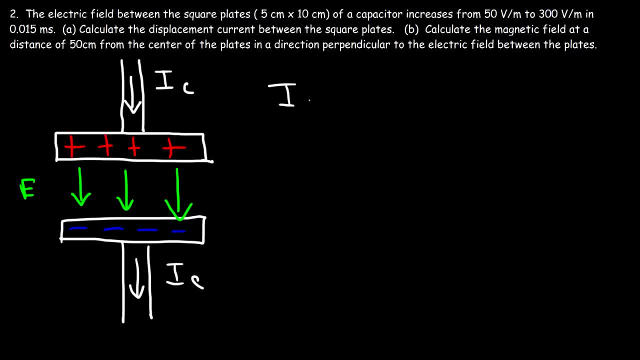 To calculate the displacement current. here's the formula that you need. It's equal to the permittivity of free space times, the rate of change of the electric flux. Now the electric flux is equal to the electric field times the area. So the electric field is changing, but the area is not. 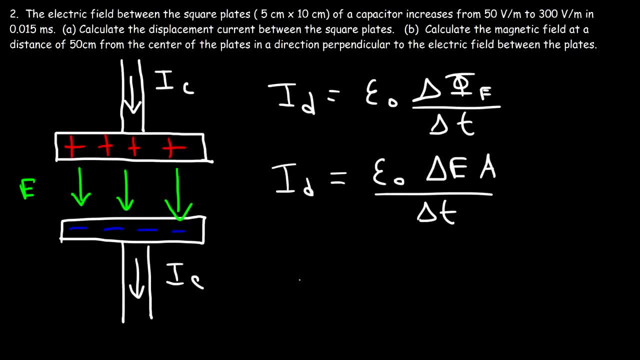 So we can use this to calculate the displacement current Now the permittivity of free space. that's 8.85 times 10 to the minus 12.. The electric field, it changes. It changes from 50 to 300.. 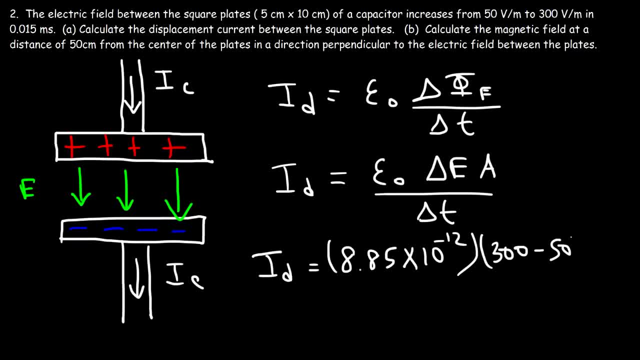 So the final amount is 300, the initial amount is 50. So the change is 250.. And then the area between the plates. that's 5 centimeters by 10.. That is the area of the plates, not between the plates. 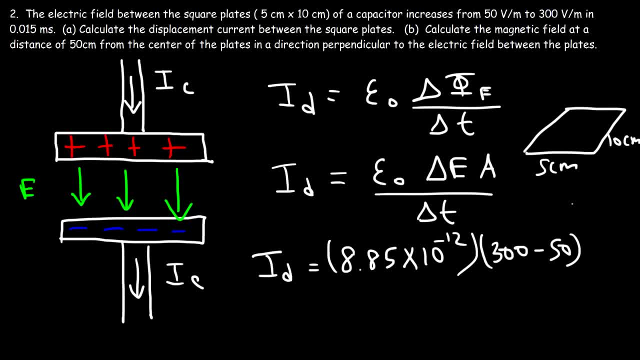 So it's 5 by 10.. 5 centimeters is 0.05 meters, And we need to multiply that by 0.1 meters, which is the same as 10 centimeters, So the area is 0.005 square meters. 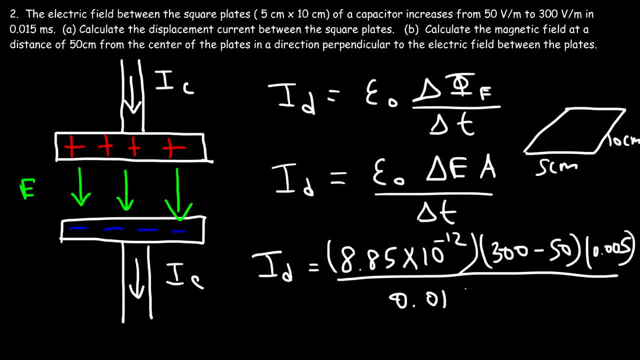 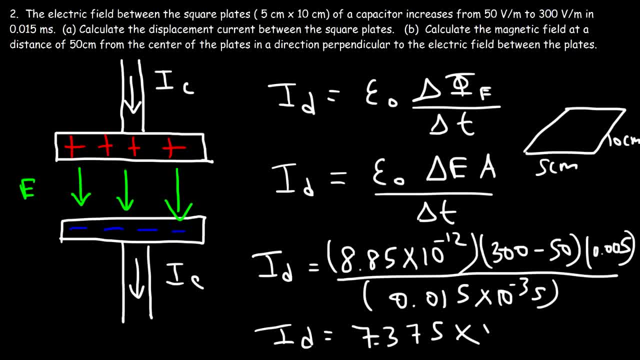 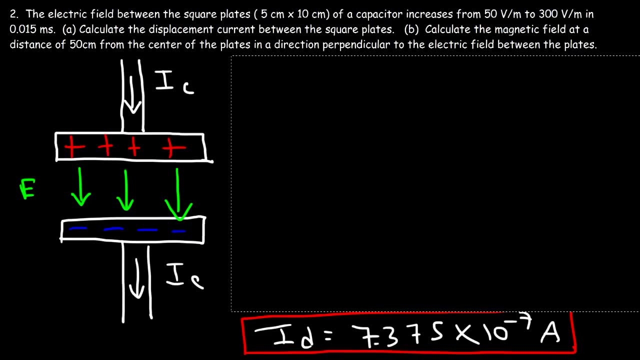 So you should get 7.35.. So you should get 7.35 times 10 to the minus 7 amps for the displacement current in between the square plates of the capacitor. And so that's how you can calculate it. Now let's move on to part B. 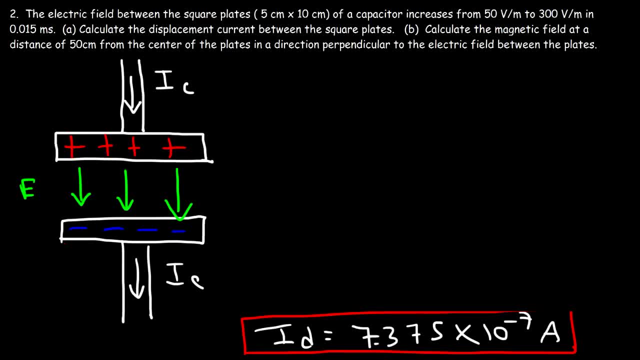 Calculate the magnetic field at a distance of 50 centimeters from the center of the plates in a direction perpendicular to the electric field. So the electric field is in the Y direction. Let's move in the X direction. So let's say this is some distance R. 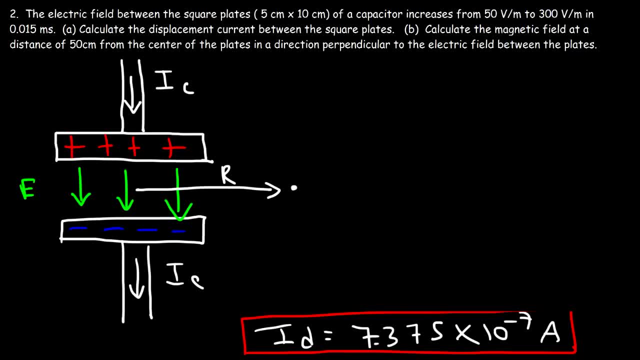 And we wish to calculate the magnetic field at this point Now. it's important to understand that if you have a current flowing in a wire in this direction, it will create a magnetic field that basically flows around the wire, And so that's the conduction current. 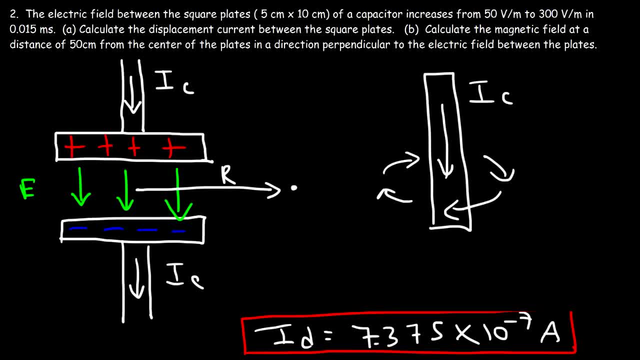 If you have a displacement current or a change in electric field, it can also induce a magnetic field, And so this magnetic field is going to be flowing around the electric field as well. So this fictitious displacement current does have an effect, And that is that a change in electric field can produce a magnetic field. 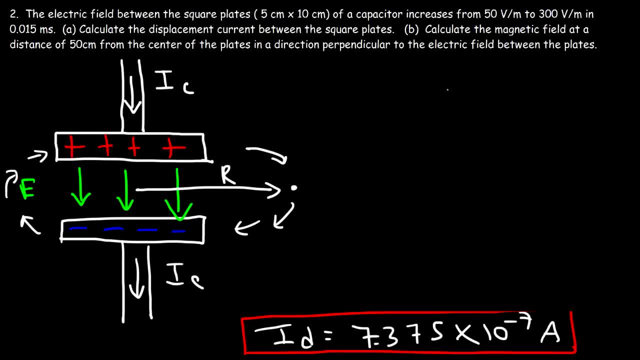 field around it. Now let's use Ampere's Law to calculate the magnetic field at this point. So we have the magnetic field times the distance that it travels, which is basically the circumference of a circle. That's 2 pi r, where the distance from the center is the. 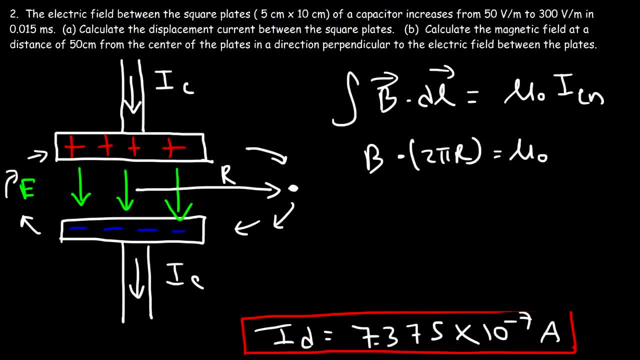 radius of the circle, And in this case the enclosed current in this region is the displacement current. The conduction current is outside of that region, And so the magnetic field is going to be mu 0 times the displacement current divided by 2 pi r. So this equation- 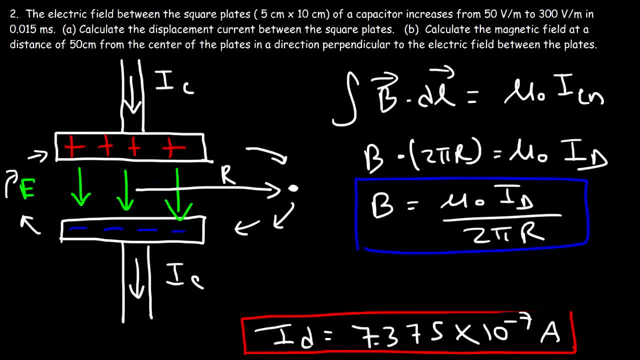 applies if you want to calculate the magnetic field where you're far outside of anywhere in between the two plates. If you wish to calculate the magnetic field somewhere in this region, it's a different equation, But outside of that region it simplifies to this equation. Notice that it's very similar to the magnetic field that flows around a. 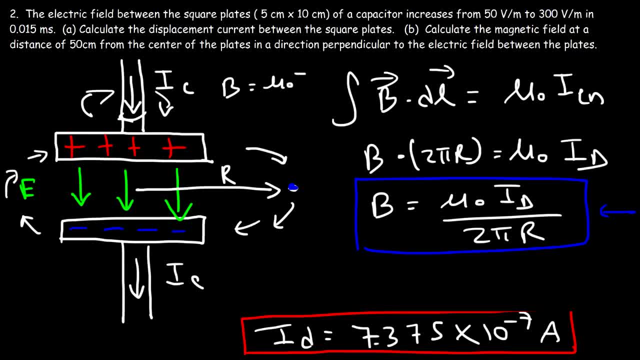 wire, which is equal to mu 0, i divided by 2 pi r. Now let's go ahead and finish this problem. So mu 0, the permeability of free space, that's 4 pi times 10 to the minus 7.. We already 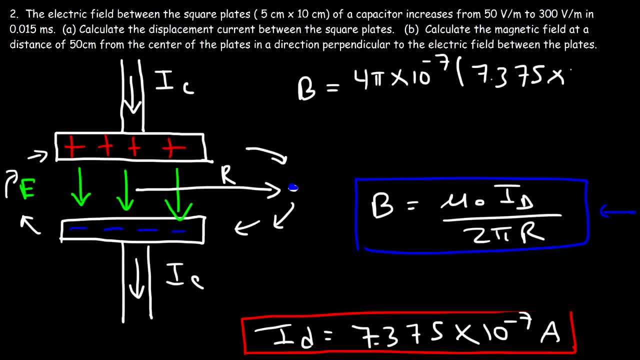 have the displacement current And the radius or the distance from the center to the point of interest. that's 50 centimeters or 0.5 meters. So 4 pi divided by 2 pi r is the displacement current And the radius or the distance from. 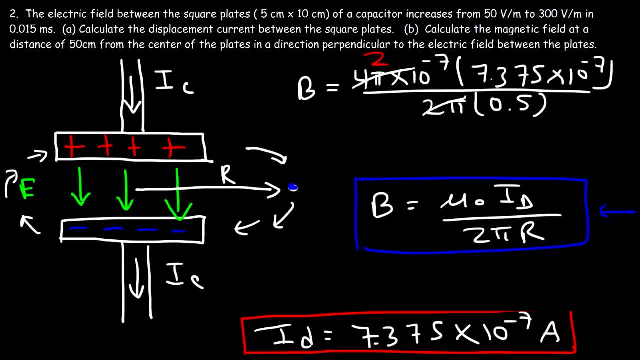 the center to the point of interest, that's 50 centimeters or 0.5 meters. So mu 0 times 10 to the minus 7 times 7.375 times 10 to the minus 7 divided by 0.5.. So the magnetic. 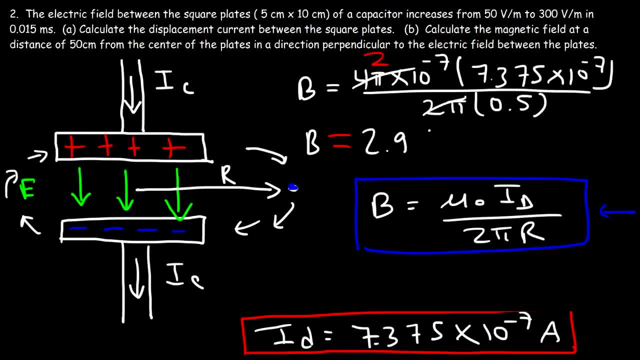 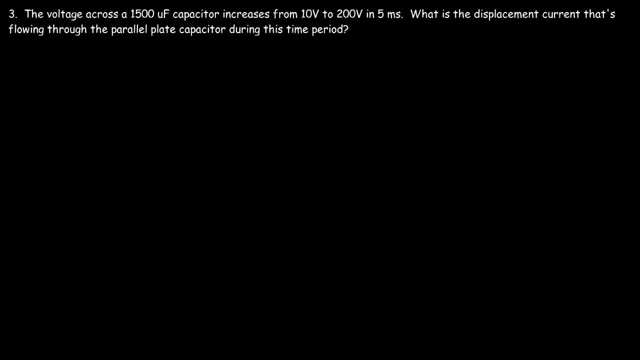 field is going to be 2.95 times 10 to the minus 13 tesla. So it's very, very small, But that's the answer: 0.5 meters. Number 3. The voltage across a 1500 microfarad capacitor increases from 10 volts to 200 volts. 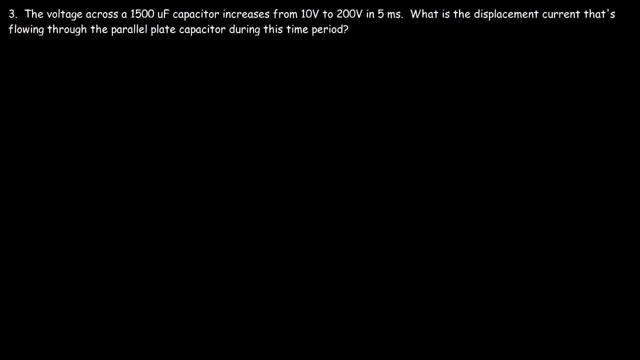 in 5 milliseconds. What is the displacement current that's flowing through the parallel plate capacitor during this time period? So how can we find the answer in this example? Well, let's start with the formula that we know. So the displacement current is the displacement current that's flowing through the parallel plate capacitor during this time period. 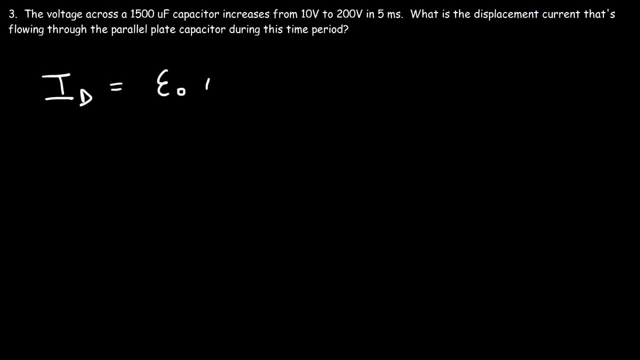 The displacement current is equal to the permittivity of free space times, the rate of change of the electric flux, And we know that the electric flux is simply the product of the electric field times the area. So we have a change in the electric field times, the area divided. 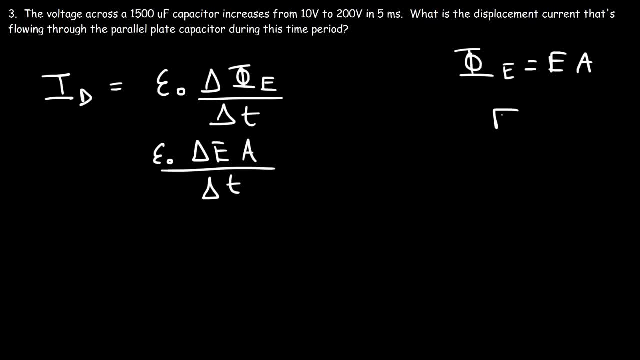 by the time Now, the electric field is the voltage across the plates divided by the distance between the plates. So the electric field times the displacement, or the distance rather, is equal to the voltage. So the change in the electric field times the 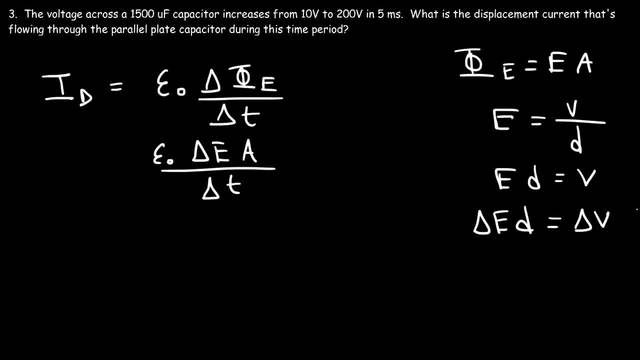 distance between the plates is equal to the change in the voltage. So what I'm going to do now is I'm going to multiply the top and the bottom by D. Now it's also important to understand that the capacitance of an air-filled capacitor 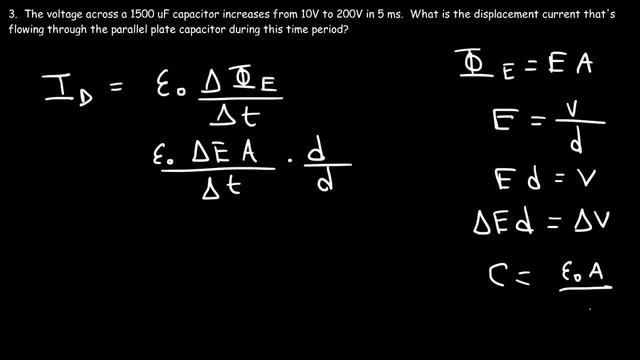 is the permittivity of free space times, the area divided by the distance. So what I'm going to do is separate these three parts. So that's going to be that times A divided by D, and then I'm going to separate these two, So delta A times D. 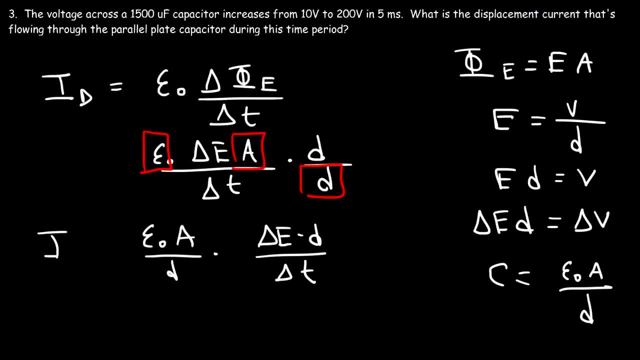 divided by D, So we can replace the permittivity of free space times the area divided by the distance with the capacitance and then the change in the electric field times the distance. I'm going to replace that with the change in voltage, So the displacement current inside a capacitor is equal to the 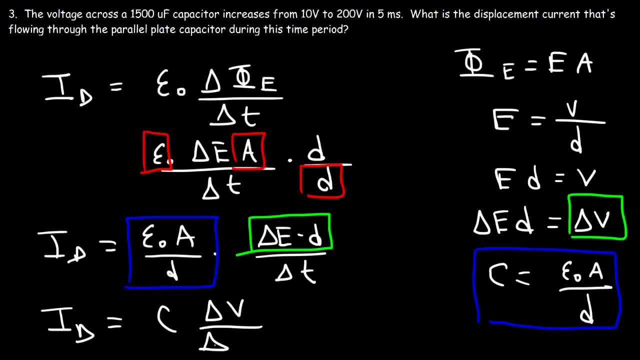 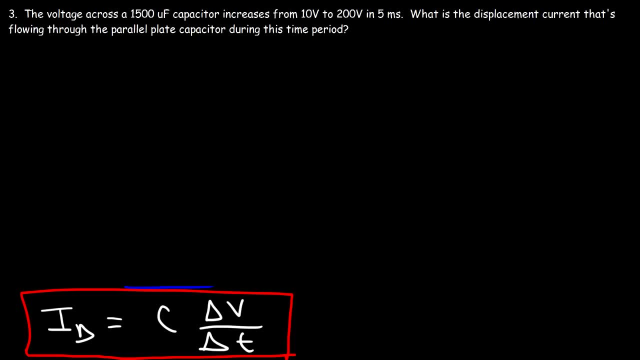 capacitance times the rate at which the voltage is changing. So this is the formula for the current displacement. So the current displacement is equal to the current displacement times the rate at which the voltage is changing. So this is the formula that we want to use in this example. 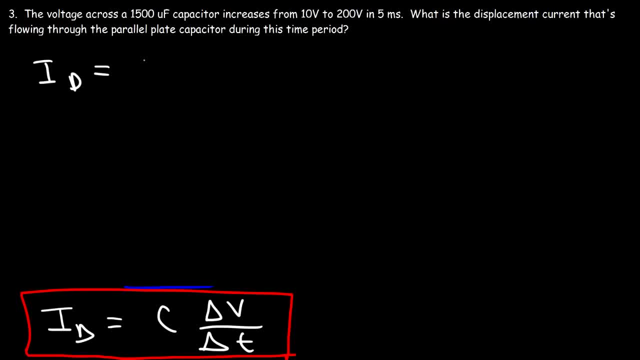 So the displacement current in this example is going to be the capacitance, which is 1500 microfarads, or 1500 times 10 to the minus 6 farads, And the voltage is equal to the current displacement times, the rate at which the voltage is changing. So this is the formula that we want to use in this example. 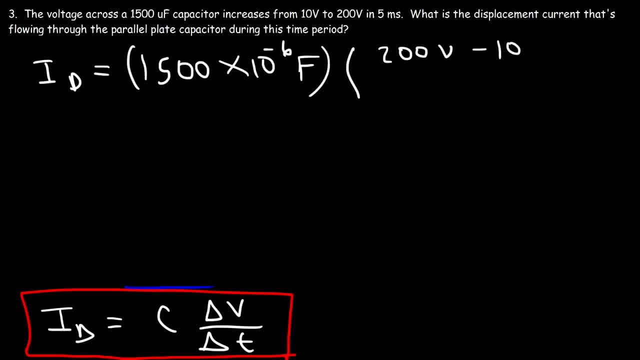 So the displacement current is equal to the capacitance, which is named after this variable. The change in voltage is 190. it's 10 minus, I mean 200 minus 10.. And then the change in time is five milliseconds, or five times 10 to minus three. 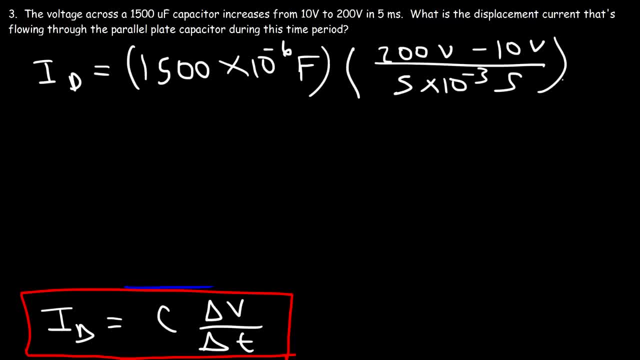 So it's gonna be 1500 times 10 minus 6 times 190, divided by 5 times 10 to the minus 3.. So the displacement current is pretty huge. in this example It is 57 amps, And so that's the answer for this problem. 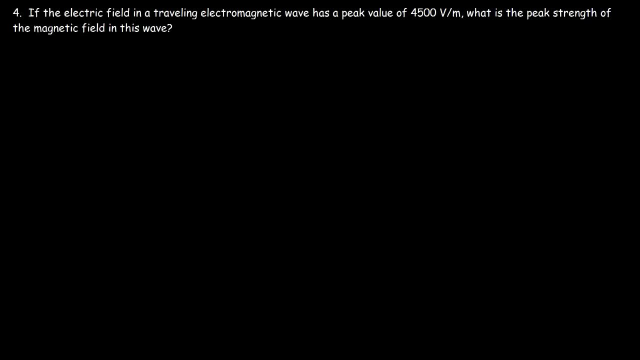 Number four: if the electric field in a traveling electromagnetic wave has a peak value of 4500 volts per meter or newtons per coulomb, what is the peak strength of the magnetic field in this wave? So let's talk about electromagnetic waves. 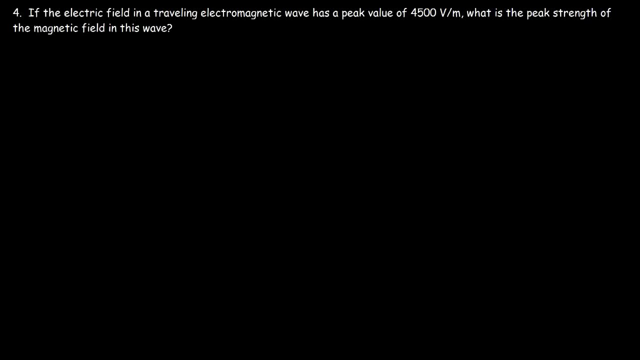 So these include light waves, x-rays, radio waves, microwaves, infrared, ultraviolet, gamma rays, all the waves in the electromagnetic spectrum, And each electromagnetic wave has an electric field component, which I'm going to draw along the y-axis. 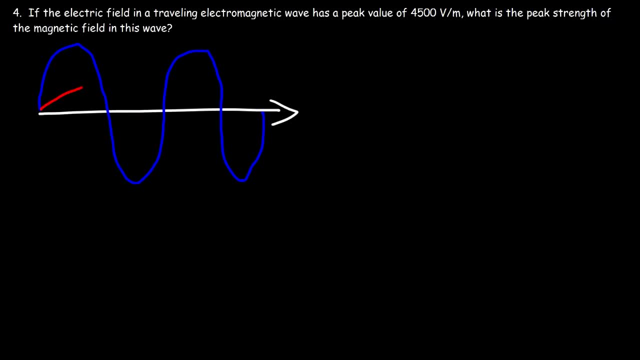 And it also has a magnetic field component which I'm going to draw along the y-axis. So you need to realize that these two are perpendicular to each other: The electric field which is in the y-direction, and the magnetic field which could be in. 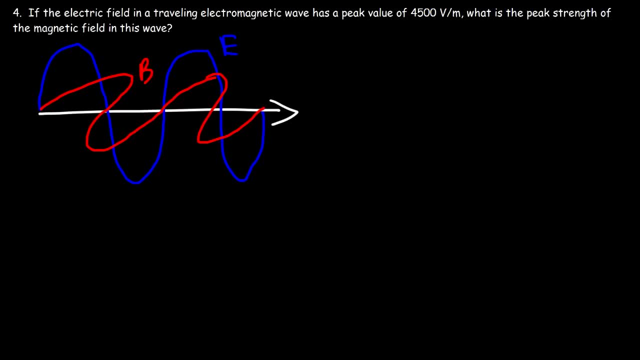 the x-direction, or sometimes in the z-direction, But these two are always perpendicular to each other, And that's what you want to take from this. Now, what's the relationship between the peak value of the electric field and the peak value of the magnetic field? 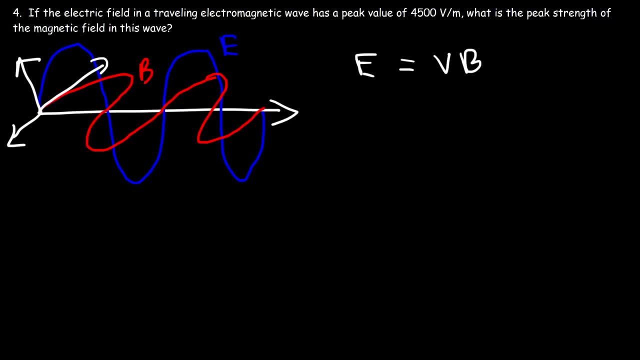 You need to know this equation: E is equal to VB. V is the speed of the traveling wave. In this case it's the speed of light. So you could say E is equal to CB, So the electric field is 4500.. 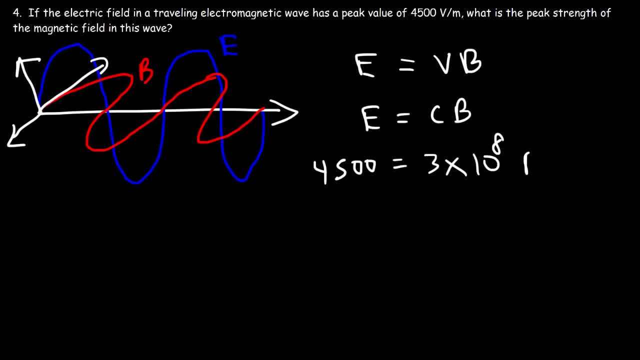 The speed of light is 3 times 10 to the 8 meters per second, And so B is going to be 4500 divided by 3 times 10 to the 8.. So the strength of the magnetic field is 1.5 times 10 to the minus 5 tesla. 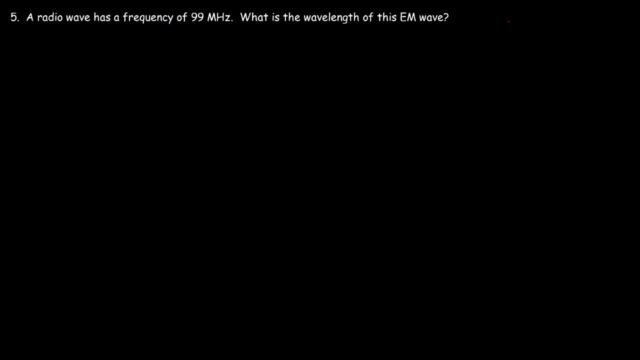 And that's the answer Number 5.. A radio wave has a frequency of 99 megahertz. What is the wavelength of this EM wave? What is the wavelength of this EM wave? What is the wavelength of this EM wave? The wavelength times the frequency is equal to the speed of light. 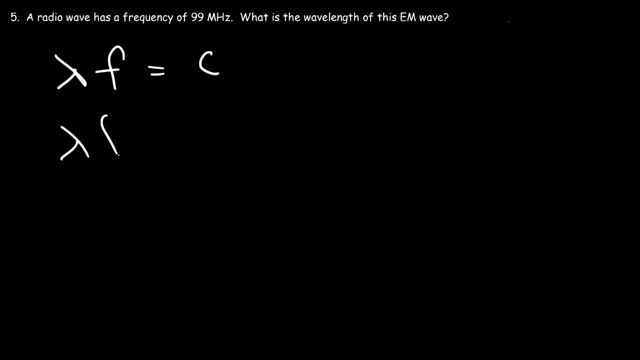 So our goal is to calculate lambda the wavelength, The frequency is 99 megahertz And mega represents 10 to the 6. Mega is basically 1 million And C the speed of light. that's 3 times 10 to the 8 meters per second. 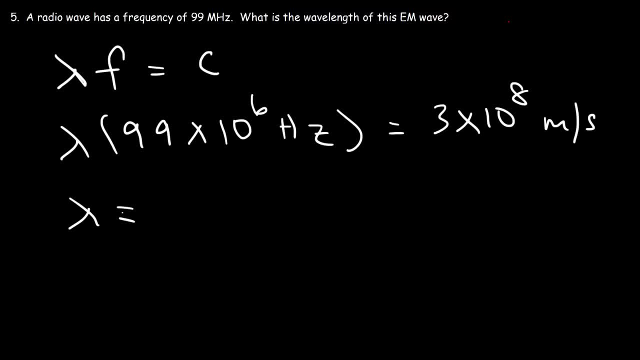 So the wavelength is the speed of light divided by the frequency, And so the wavelength is going to be about 3.03 meters. So that is the length of the wave that has a frequency of 99 megahertz, And so that's it for this problem. 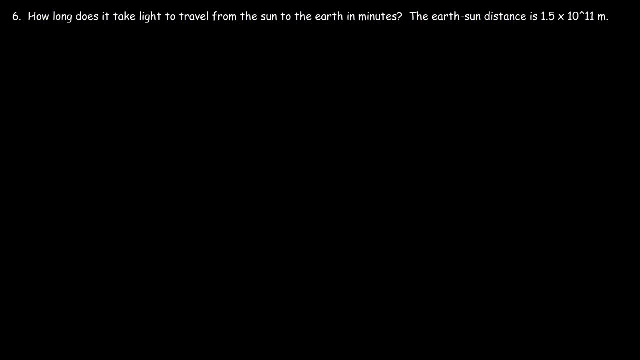 Number 6. How long does it take light to travel from the sun to the earth? in minutes. So let's say this is the sun And here we have the earth. So how long does it take light to travel from the sun to the earth? 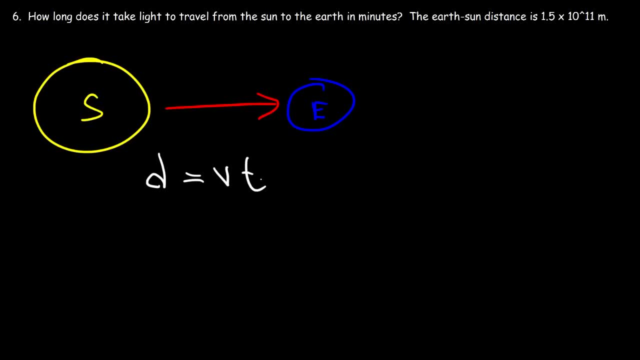 So we could use this formula. d is equal to vt. So the distance between the sun and the earth, that's 1.5 times 10 to the 11 meters. The speed at which light travels is 3 times 10 to the 8 meters per second. 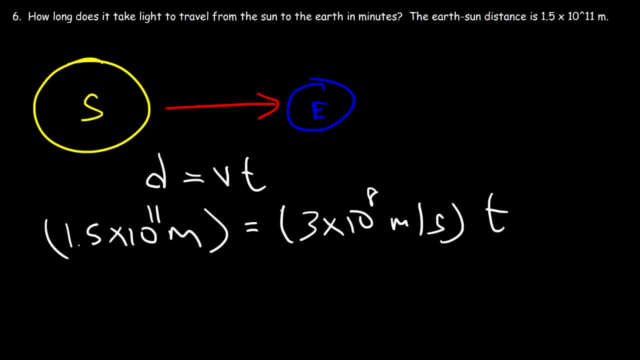 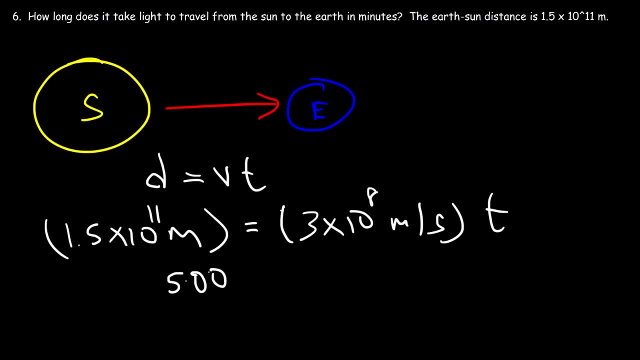 1.5 times 10 to the 8 meters per second, And so this is going to be 500.. And so this is going to be 500.. Now we can see that the unit meters cancel, so we're left with seconds. 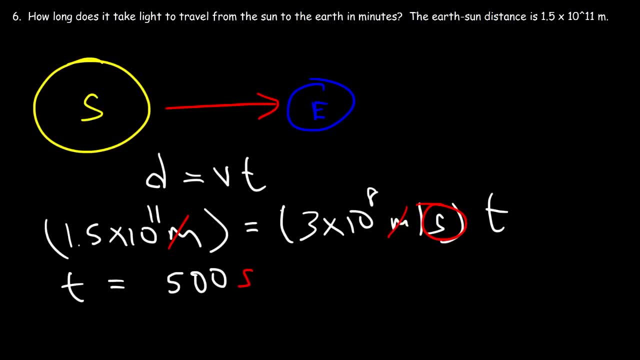 So this is 500 seconds, So that's equal to t. Now let's convert that to minutes, So 1 minute is equal to 60 seconds, And so this is about 8.3 minutes. So that's how long it takes light to travel from the earth to the sun. 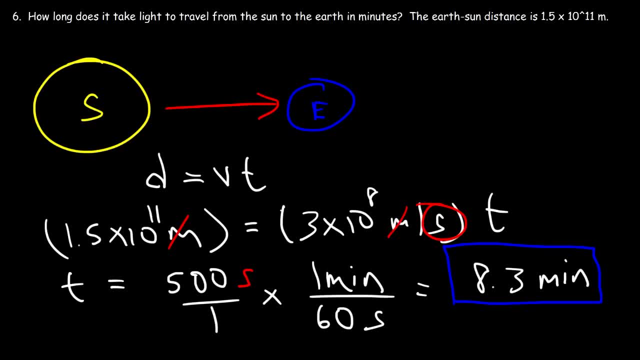 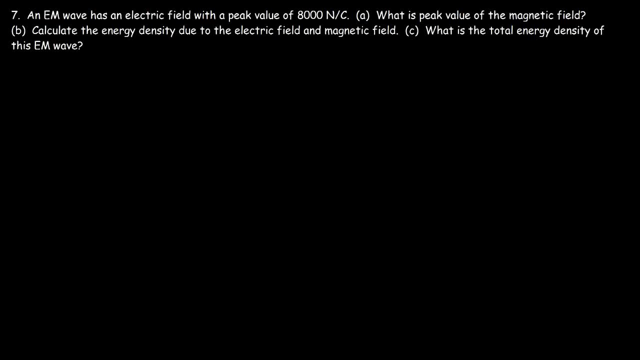 So when you're looking at the sun, you're looking at how it appeared 8 minutes ago, Number 7.. An EM wave has an electric field with a peak value of 8,000 newtons per coulomb. What is the peak value of the magnetic field? 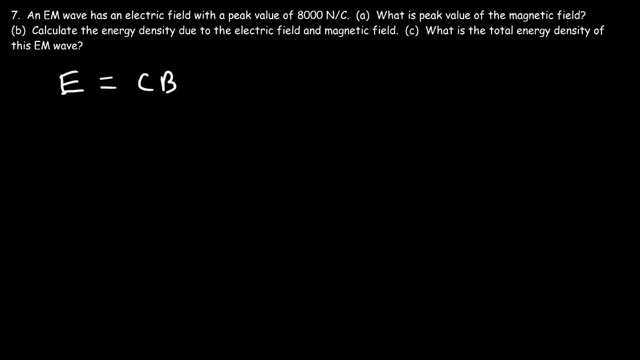 So we know that E is equal to CB. So E in this example is 8,000.. The speed of light is 3 times 10 to the 8 meters per second, And so, to calculate B, it's going to be 8,000 divided by 3 times 10 to the 8.. 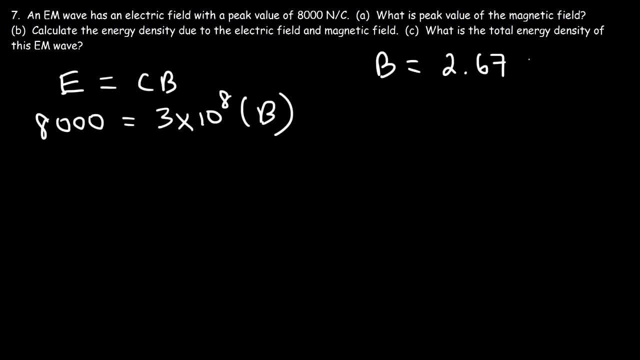 So the strength of the magnetic field is going to be 2.67 times 10 to the minus 5 Tesla. So that's it for Part A. Now Part B: Calculate the energy density due to the electric field and magnetic field. 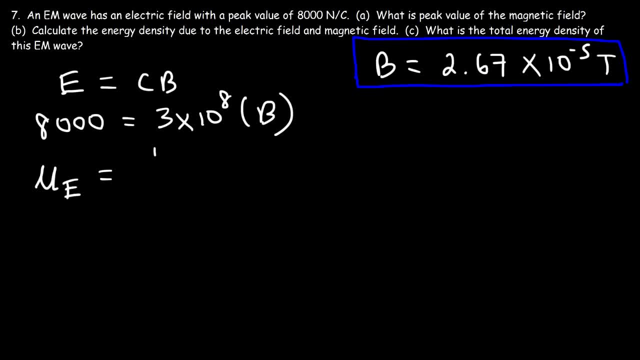 The energy density due to the electric field. It is 1 half the permittivity of free space times E squared. So that's the formula. you need to get it. Now let's go ahead and plug in everything that we know. 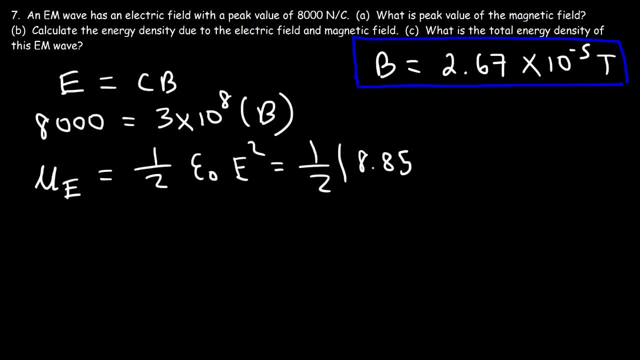 The permittivity of free space is 8.85 times 10 to the minus 12.. And in this example the electric field is 8,000 newtons per coulomb- And don't forget to square it. So the energy density due to the electric field, that's equal to 2.8 times 10 to the minus 4.. 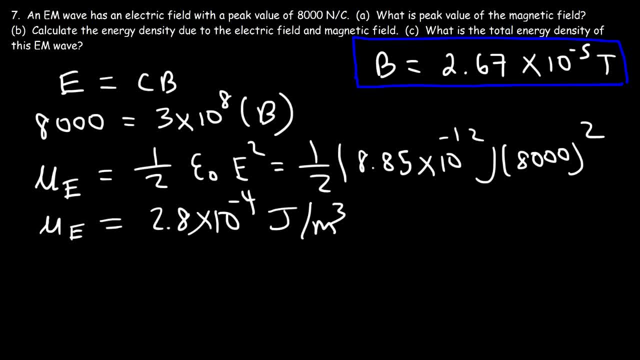 And it's joules per cubic meter. The energy density is the energy per unit volume. Now let's do the same thing for the magnetic field, And so what is the formula that we need in order to calculate the energy density due to the electric field? 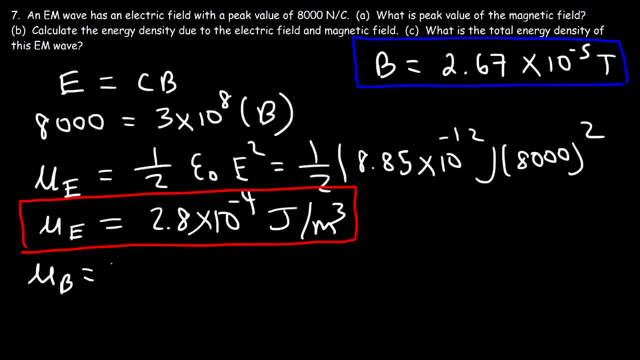 Here it is. It's going to be 1 half B squared, divided by mu 0 or mu naught. So the strength of the magnetic field is 2.67 times 10 to the minus 5.. And the permittivity of free space is 4 pi times 10 to the minus 7.. 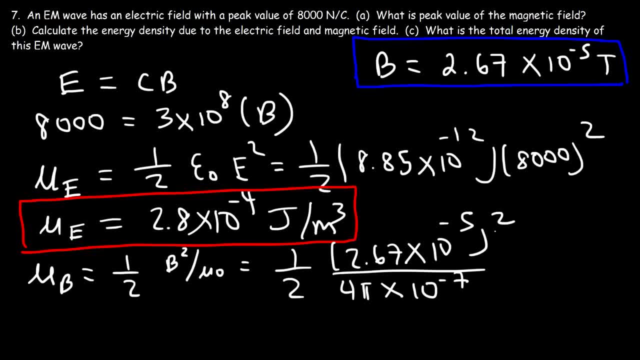 And we need to square that as well. So we need to substitute 1 half B, squared by mu, 0, 1 by mu naught, And this gives you the same answer: 2.8 times 10 to the minus 4 joules per cubic meter. 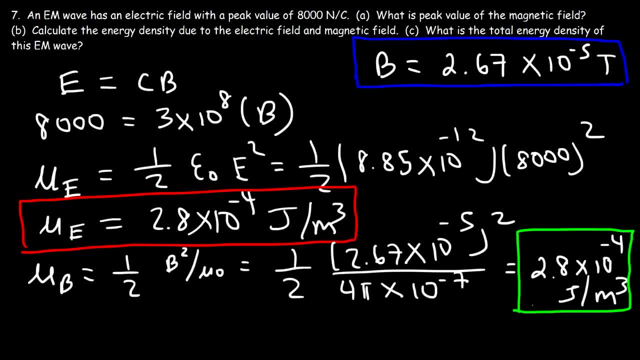 So what this tells us is that the energy density of the magnetic field and the electric field in an EM wave is the same. So the total energy density of the EM wave is 2.8 times 10 to the minus 4.. 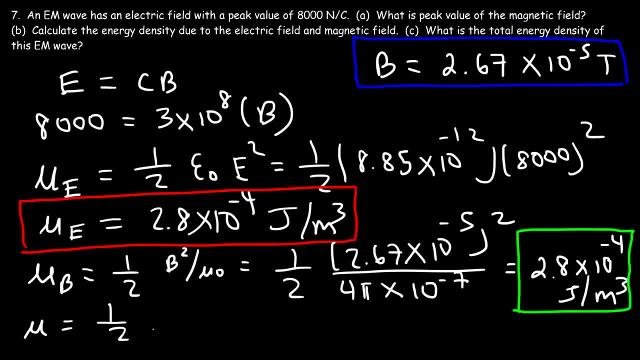 So what this tells us is that the energy density of the magnetic field and the electric field in an EM wave is the same. It's going to be the sum of the contributions for the electric field. So it's 1 half epsilon naught times e, squared plus the contribution from the magnetic field. 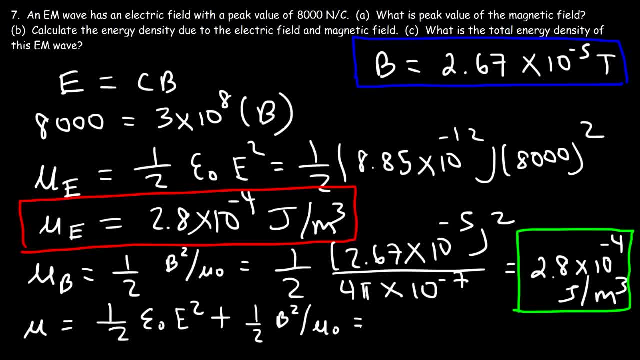 1 half b squared, divided by mu naught, And so it's basically this number times 2.. So this is going to be approximately 5.6 times 10 to the minus 4 joules per cubic meter. And keep in mind these values are rounded, so this is also going to be a rounded answer. 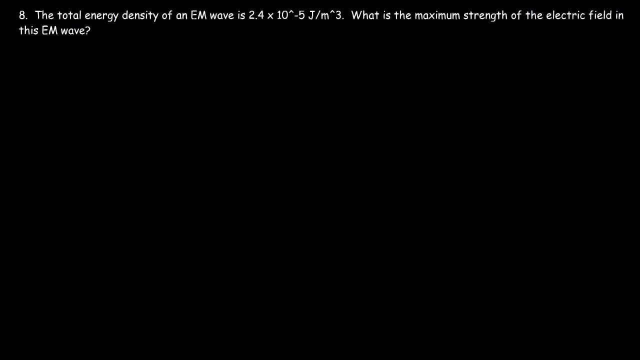 So it's approximately equal to that Number 8.. The total energy density of an EM wave is 2.4 times 10 to the minus 5 joules per cubic meter. What is the maximum strength of the electric field in this EM wave? 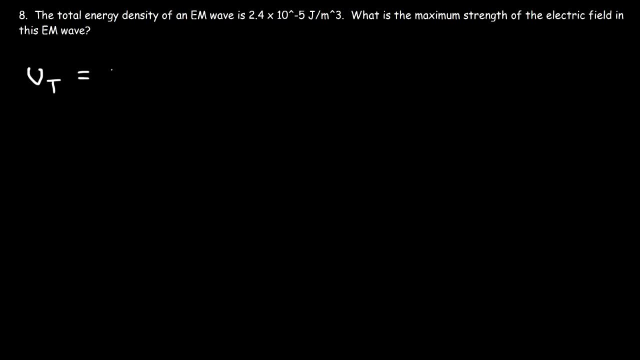 So we saw that the total energy density is The energy density of the electric field plus the energy density of the magnetic field. So the energy density due to the electric field is 1 half epsilon, naught times the square of the maximum electric field. 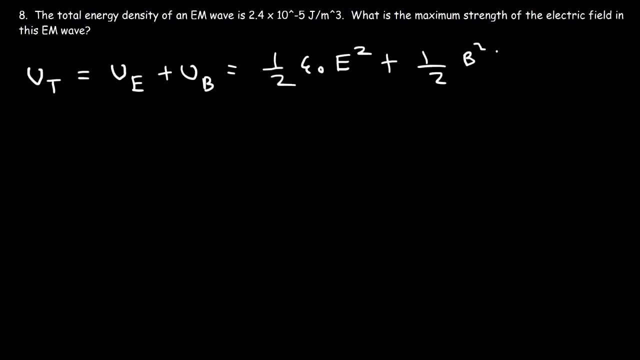 And then it's 1 half times b squared, divided by mu zero. Now we also saw that in the last problem the energy density of the electric field and the magnetic field were equal. So therefore, what I can do is I can replace this with the energy density of the electric field. 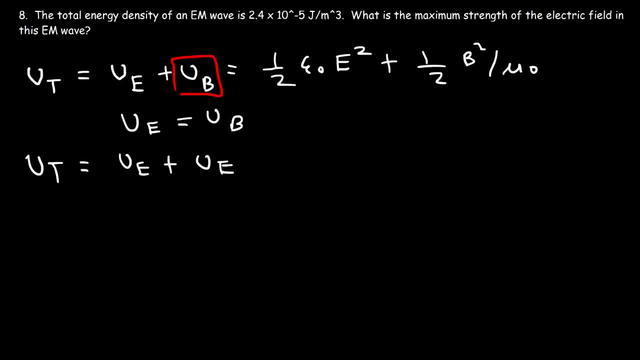 Since they equal each other. So I have 1 half epsilon naught e squared plus another 1 half epsilon naught e squared. 1 half plus 1 half is a whole. So the total energy density That's a lowercase u, by the way. 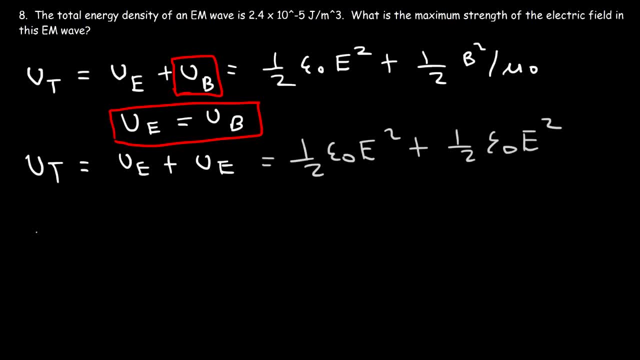 Not a capital U. The total energy density of an EM wave, in terms of the electric field only, is simply equal to 1 epsilon naught e squared. So we have the total energy density, That's 2.4 times 10 to the minus 5.. 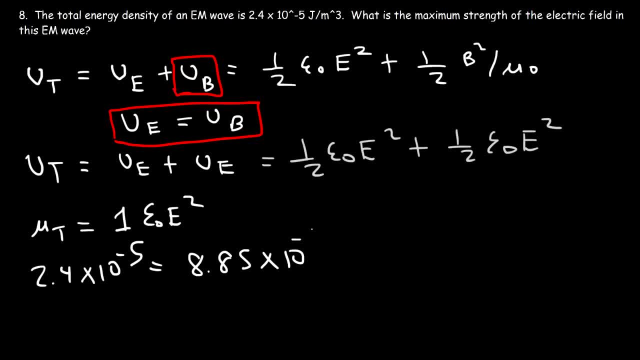 Epsilon naught is 8.85 times 10 to the minus 12.. And so let's calculate the strength of the electric field. So the strength of the electric field is going to be 1647 newtons per coulomb, or volts per meter. 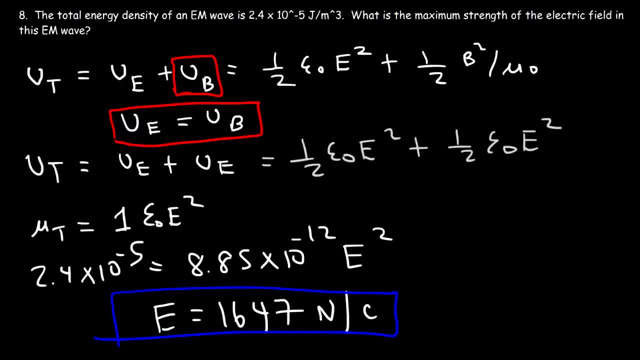 So that's the answer. Now don't forget, after you divide the total energy density by epsilon naught, don't forget to take the square root, because we have an e squared. So after you take the square root, you should get the final answer of 1647.. 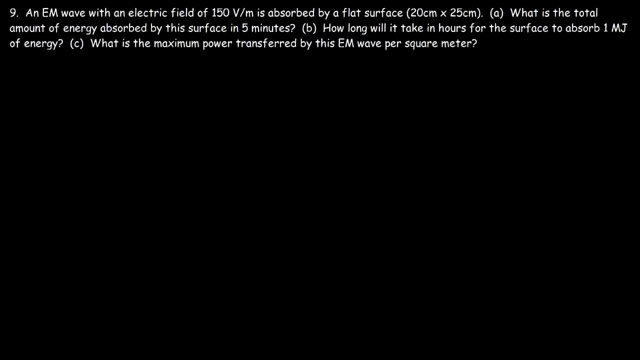 Number 9. An EM wave with an electric field of 150 volts per meter is absorbed by a flat surface. So let's draw a picture, Let's say this is the flat surface. So let's say it looks something like that, And so this is the area of the flat surface. 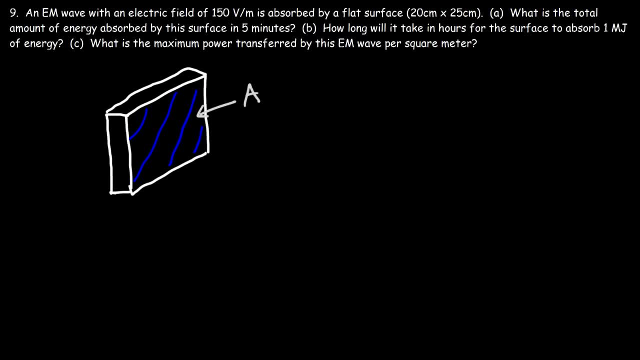 We'll call it A And let's say this is the EM wave that's traveling towards it. Let's say this is the magnetic field And this is the electric field of the EM wave, And this is going to be called delta x. 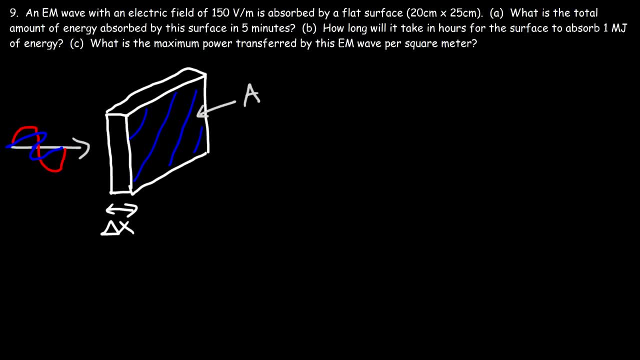 That's the electric field And this is the width of the surface. So what is the total amount of energy absorbed by this surface in 5 minutes? So this surface has a length of 20 centimeters and a width of 25 centimeters. 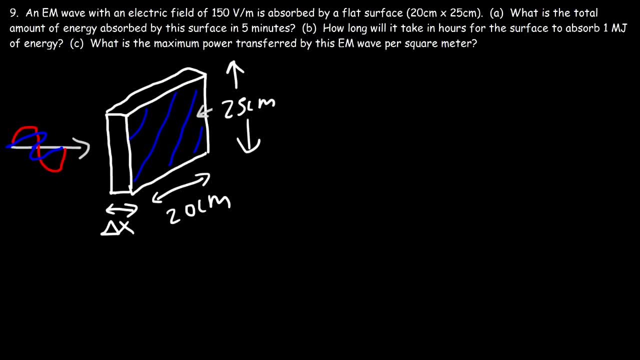 With this information, how can we calculate the total amount of energy absorbed by this surface, The total energy which we're going to use? capital U for potential energy? that's going to equal the energy density lowercase u times the volume. Energy density is joules per cubic meter. 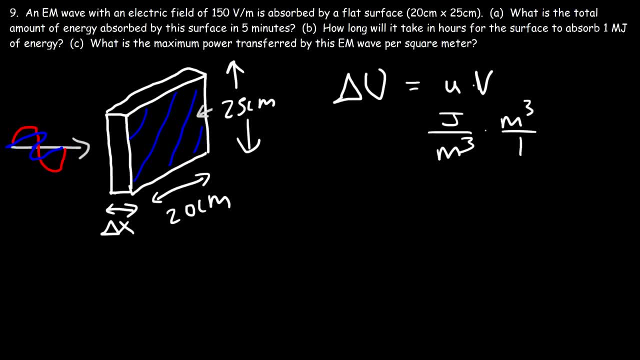 If we multiply that by the volume in cubic meter, then we'll get the energy stored in joules. Now the energy density of an EM wave in terms of the electric field is epsilon naught times e squared. Now, keep in mind, this value includes the strength of the electric field and the magnetic field. 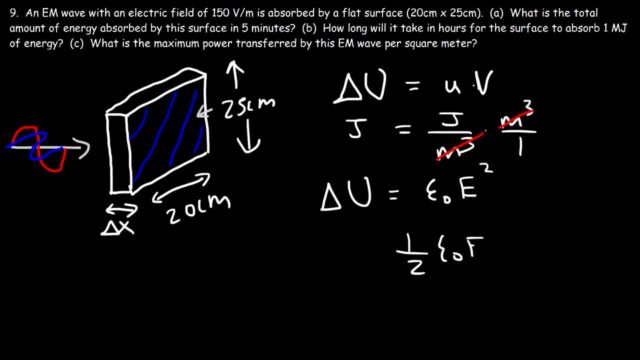 If it's just the electric field alone, it's one half, But then plus the magnetic field it's another one half. epsilon zero, e squared, So this gives us the total total energy density for the entire EM wave in terms of the electric field alone. 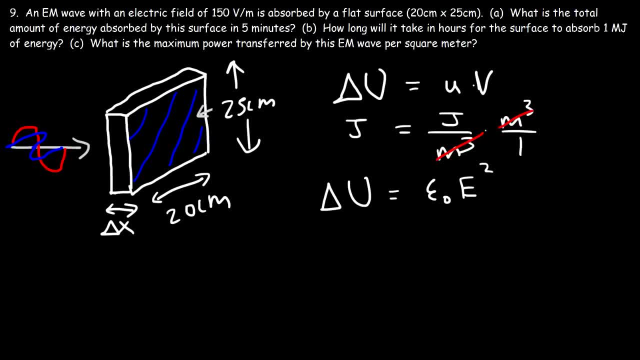 So just keep that in mind. So that's the energy density of the EM wave multiplied by the volume. So the volume is going to be delta X times the area. Now, what is delta X? Delta X represents the distance, and distance is equal to velocity multiplied by time. 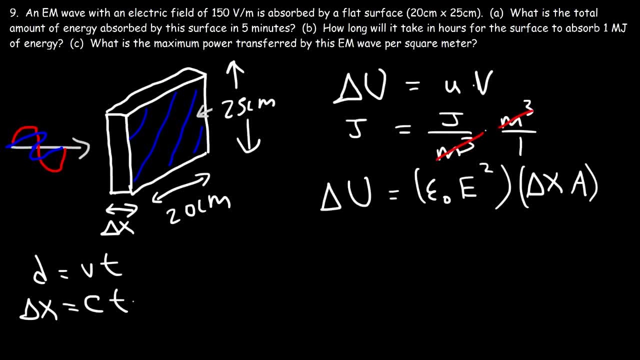 So we can replace delta X with the speed of light times the time that it takes to pass through the surface. So thus we have this equation, So CT times A. So the final equation that we can put all together is that the energy that's going 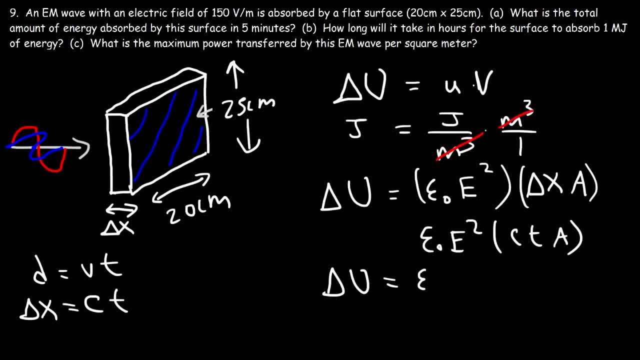 to be absorbed by the flat surface is equal to epsilon naught times the speed of light, times E squared times the area multiplied by the time. So this is the formula that you want to write down. So now let's focus on part A. So epsilon sub zero, that's 8.85.. 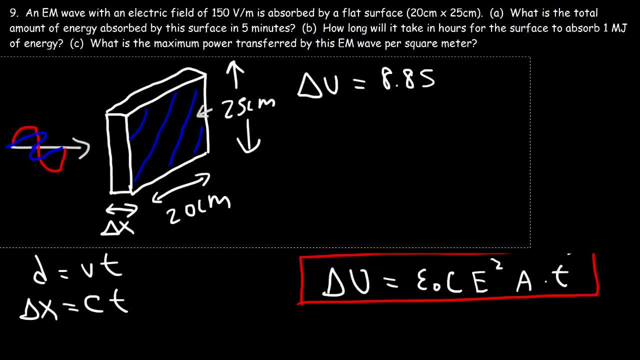 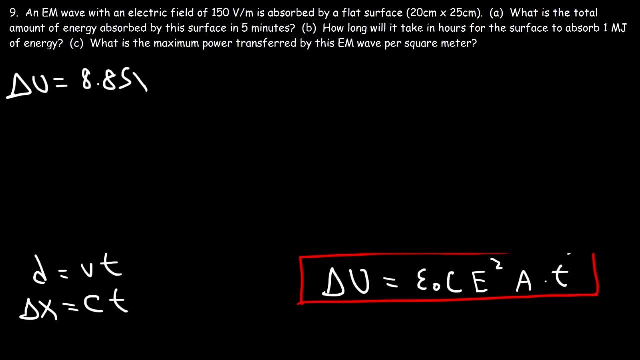 So actually, let me get rid of this now. You can always just rewind if you need that picture again. So epsilon sub naught, that's 8.85 times 10 to the minus 12.. And then we have the speed of light: 3 times 10 to the 8 meters per second. 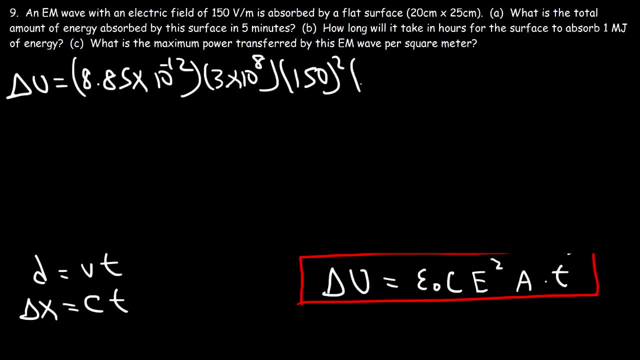 And the electric field. that's 150 volts per meter. The area is going to be just those two multiplied to each other in meters. 20 centimeters is 0.2 meters, So that's 0.2 meters. 25 centimeters is 0.25 meters. 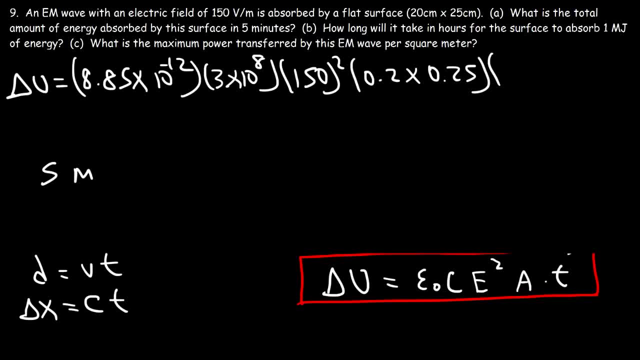 And the time is 5 minutes. So let's convert that to seconds. So we know that there's 60 seconds per minute, And so 5 times 60 is 300 seconds. So go ahead and plug those numbers in. So the total energy transferred to the flat surface in 5 minutes is 896 joules. 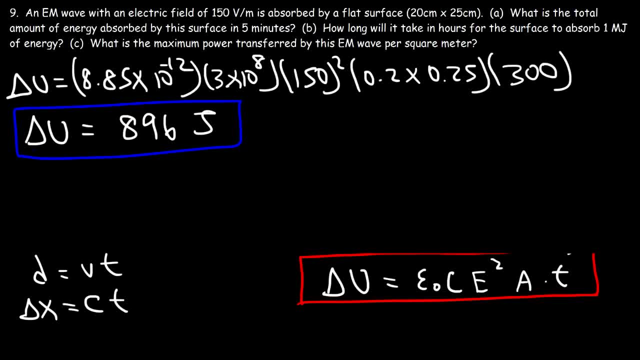 And so that's the answer for part A. Now part B. how long will it take in hours for the surface to absorb 1 megajoule of energy? 1 megajoule, 1 megajoule 10 to the 6 joules? 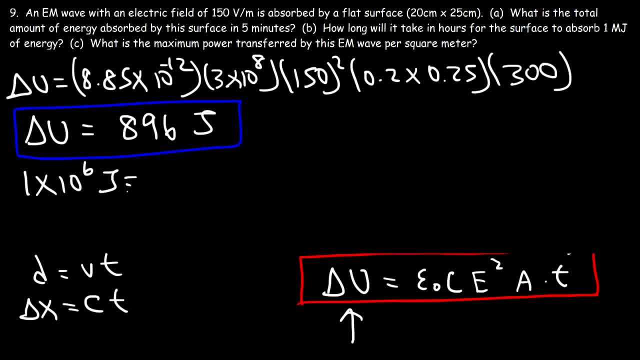 So that's a million joules, That's delta. U. Now, everything else is going to be the same except T. So epsilon, sub naught, that's the same. The speed of light, the electric field, that's going to be the same. 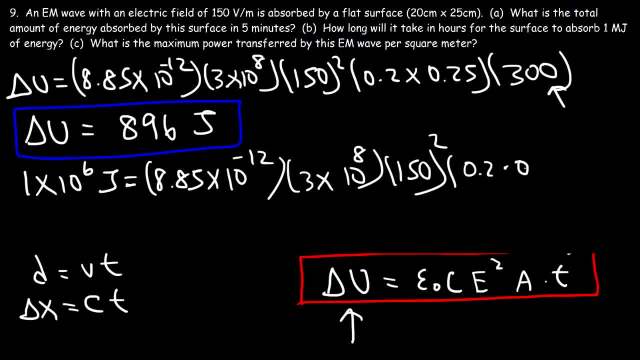 And the area is going to be the same. So let's calculate T. So first let's multiply 8.85.. And that's 10 to the 6 joules, Times 10 to the minus 12.. Times 3 times 10 to the 8.. 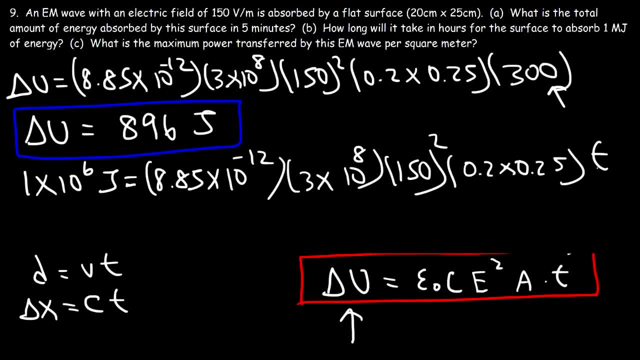 Times 150, squared Times 0.2 and 0.25.. And so that should give you 2.987 multiplied by T. So then T is going to be 1 times 10 to the 6 divided by 2.987.. 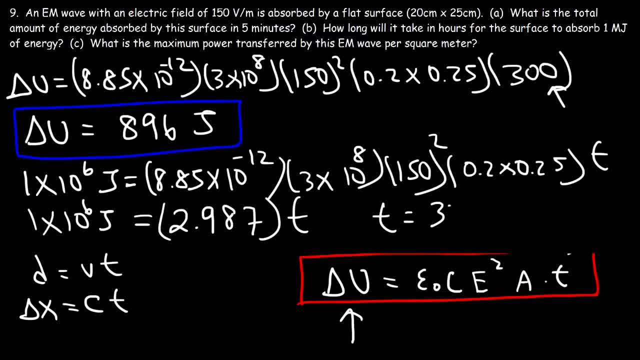 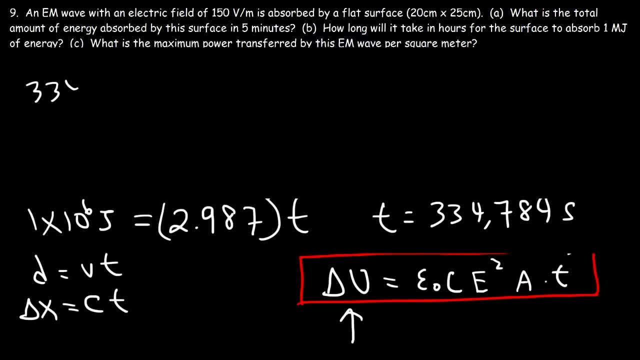 2.987.. 2.987.. The time is about 334,784 seconds, So let's go ahead and convert that answer into hours. Now the 60 seconds in one minute, and in one hour there's 60 minutes. 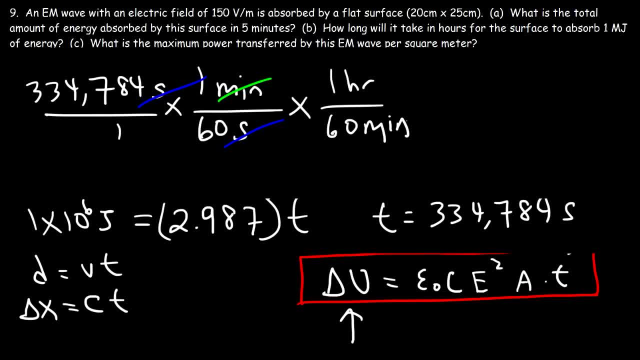 So basically we got to take our answer and divide it by 3600. So this is going to be approximately 93 hours if you round it. So that's how long it will take for this surface to absorb one megajoule of energy. 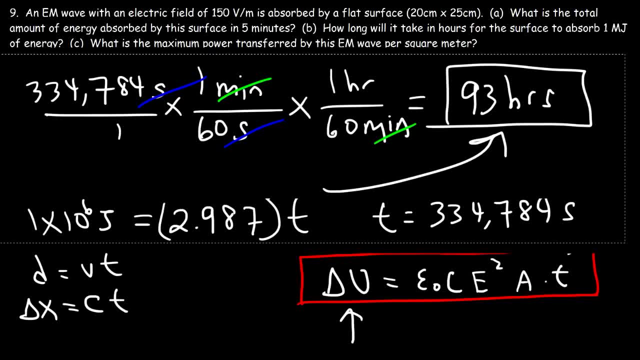 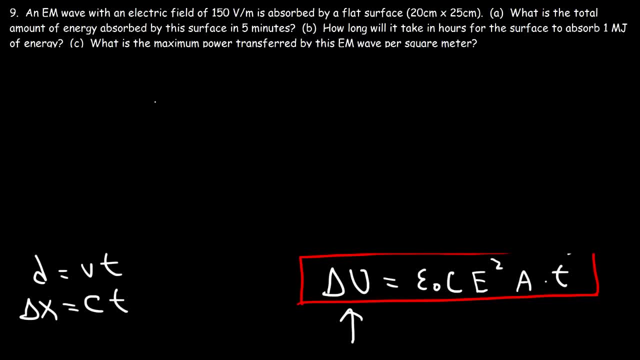 Now let's move on to part C. What is the maximum power transferred? Okay, The maximum power transferred by this EM wave per square meter Power is equal to energy divided by time. Energy is in joules, time is in seconds, and one joule per second is one watt. 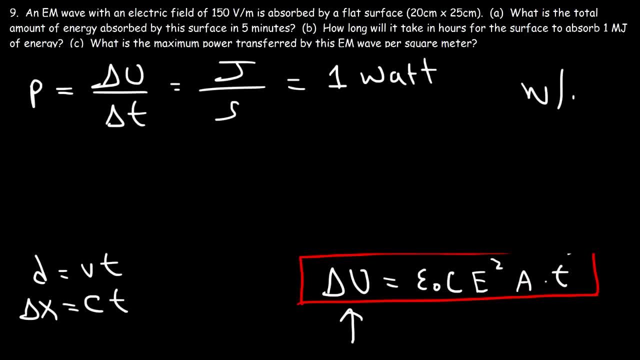 Now what we want is power per square meter, so we want watts per square meter. So that's represented by the symbol S, also known as the Poynton vector. so we want to calculate just the magnitude, The magnitude of the Poynton vector, not the direction. 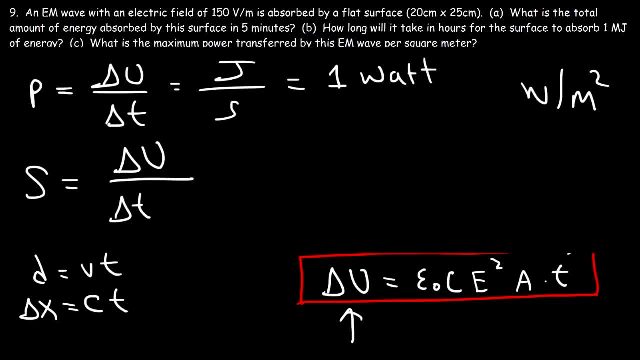 So it's going to be the energy divided by the time. so that's going to give us the power in watts, but then we need to divide it by the area in square meters. so that's A. So delta, U is this equation? 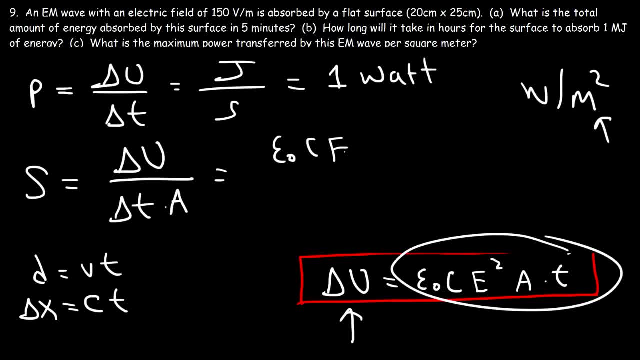 It's epsilon sub naught, C, E squared A, T, and we need to divide it by the area and by the time. So these will cancel and these will cancel. So therefore, S is going to equal. this is the maximum value of S. epsilon sub naught. 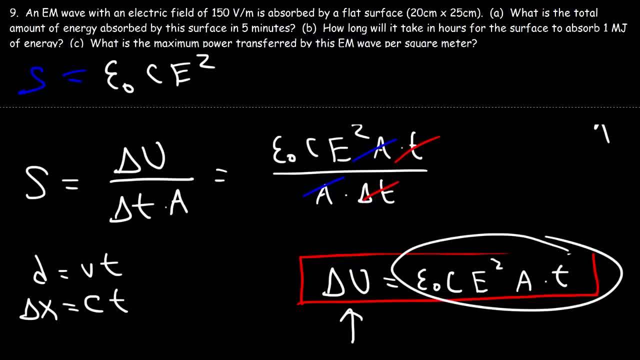 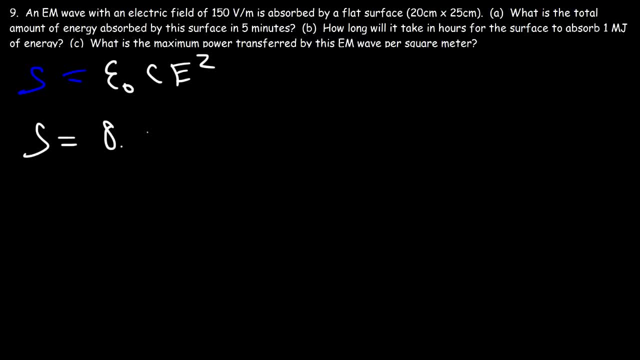 C, E squared, And so that's the formula that we need. Okay, Okay, Okay. So epsilon sub-naught is 8.85 times 10 to the minus 12.. The speed of light is 3 times 10 to the 8 meters per second. 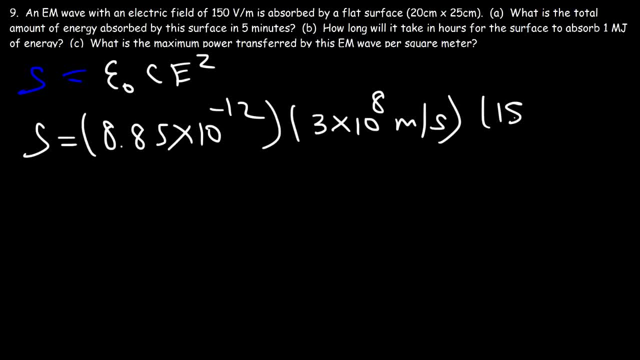 And the electric field is 150 volts per meter And we need to square it And so this is going to be 59.7 watts per square meter. So this has the same unit as intensity, which is also watts per square meter. 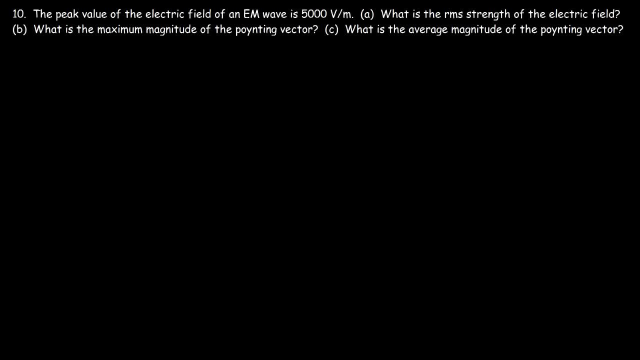 Number 10.. The peak value of the electric field of an EM wave is 5,000 volts per meter. What is the RMS strength of the electric field? The RMS strength is going to be the peak electric field divided by the square root of 2.. 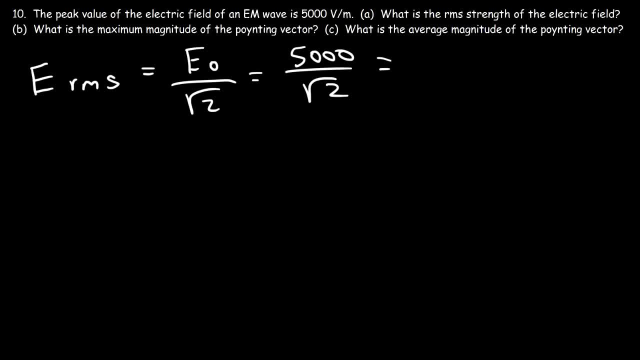 So it's 5,000 divided by the square root, And so that's going to be 3,535.5 volts per meter. Now what is the maximum magnitude of the point and vector To calculate it? it's going to be: S is equal to epsilon sub-naught CE squared. 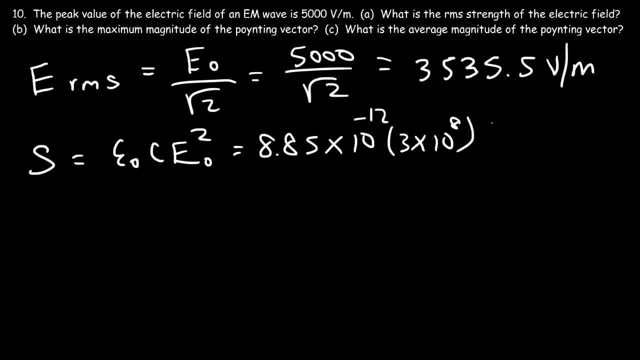 And so we need to use the peak electric field value, which is 5,000.. And so you should get 66,375 watts per square meter. So that's the power per unit area. Now, to calculate the RMS strength of the electric field, we need to use the peak electric field value, which is 5,000.. 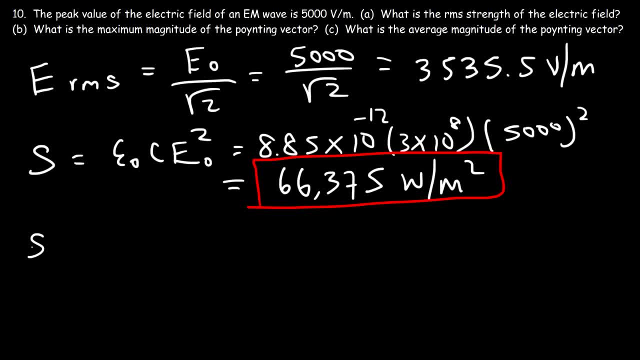 So we need to use the peak electric field value, which is 5,000.. magnitude of the points in vector: it's simply going to be 1, half of this value. so you just divide that by 2, so it's 33,000, 187.5 watts per square meter. now. 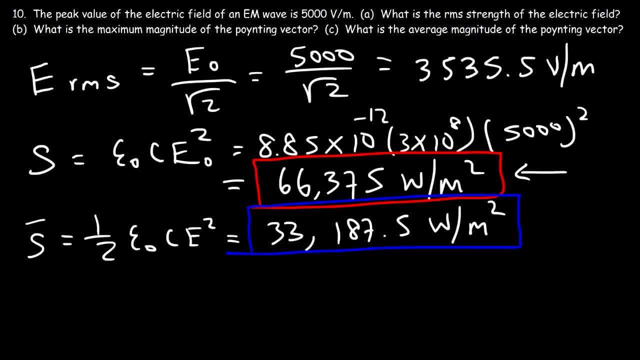 you can also get that answer if you're using the RMS value of the electric field. if you decide to use that, you no longer need the 1 half. it's going to be epsilon sub naught, C, e, RMS squared, so that's 8.85 times 10 to the minus 12. 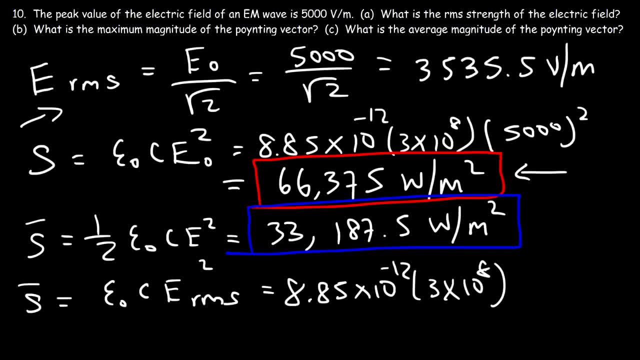 times 3, times 10, to the 8, and then times 35, 35.5 squared, and so this is going to be 33,000, 186.9 watts per square meter. so this answer is very close because I use a rounded answer, not the exact answer. so if you use the exact answer here, then 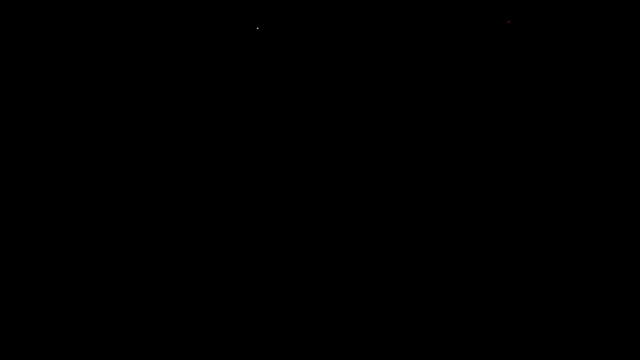 these two should be exactly the same. now here are some other formulas that you may find useful. so you've seen this one already, using the peak electric field value, but in terms of the magnetic field, you can use this equation and keep in mind: mu naught of Buons ka. delta 0 is 4. 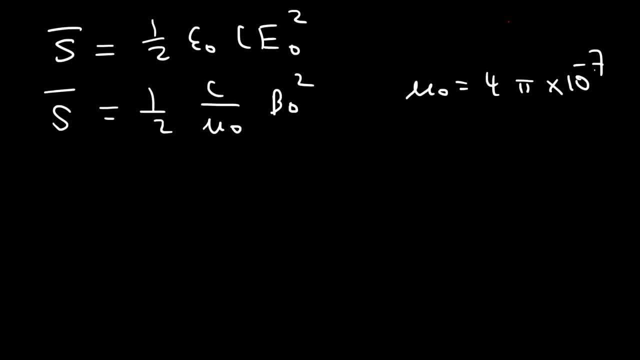 Pi times 10 to the minus 7. that's the permeability of free space. you can also use this equation if you have the peak values of the electric field and a magnetic field, or if you have the RMS values. you can use this equation, yeah, yeah. 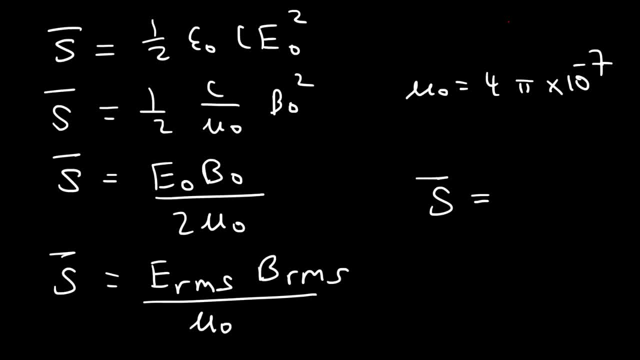 Now keep in mind the average power per square meter. that's going to be one half of the maximum value. So if you have the maximum value, you need to find the average value. just multiply by one half, And so those are some extra formulas that you need to know. 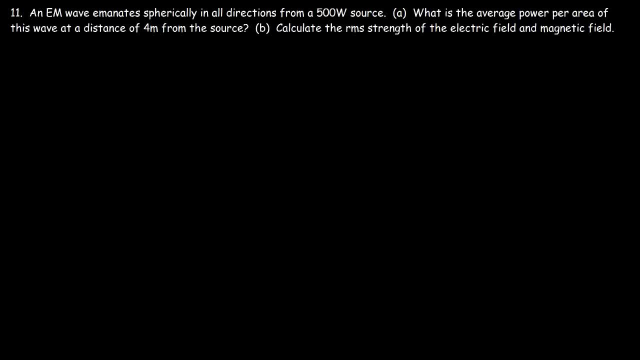 Number 11.. An EM wave emanates spherically in all directions from a 500 watt source. What is the average power per area of this wave at a distance of 4 meters from the source? So let's say if we have a source of the EM waves. 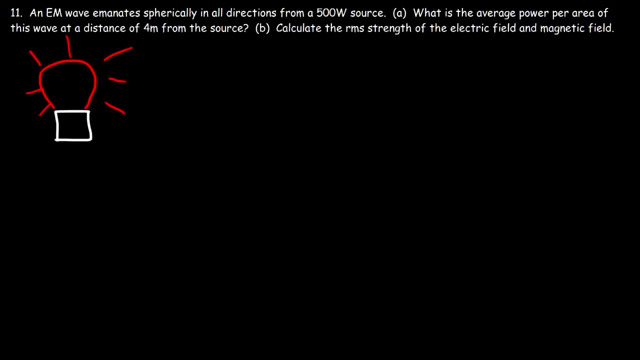 And so it emanates in all directions in the shape of a sphere. We need to find how much power, or the power per area, at a distance of 4 meters away from this Now, S is equal to the energy divided by the time, divided by the area. 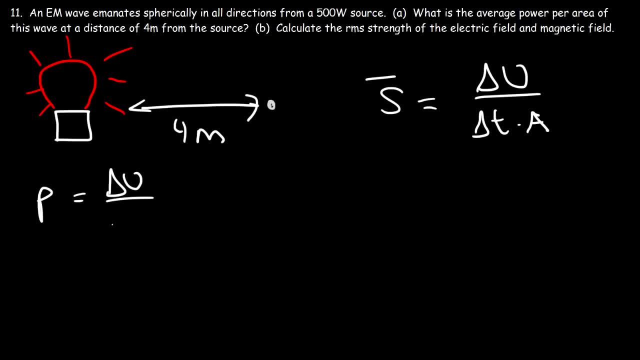 And power is energy per unit time. So we can say that S, or the average S value, is going to be the average power divided by the area, And so we have the power of the source, That's 500 watts. 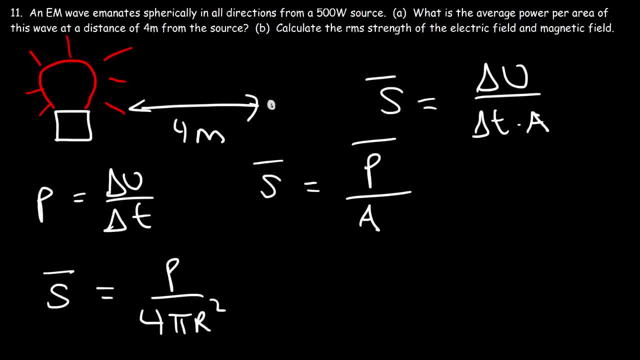 And we need to divide it by the surface area of the sphere, Because it emanates spherically in all directions. Actually, let me get rid of this whole thing. So it's going to be 500 watts divided by 4 pi, and the distance is 4 meters. 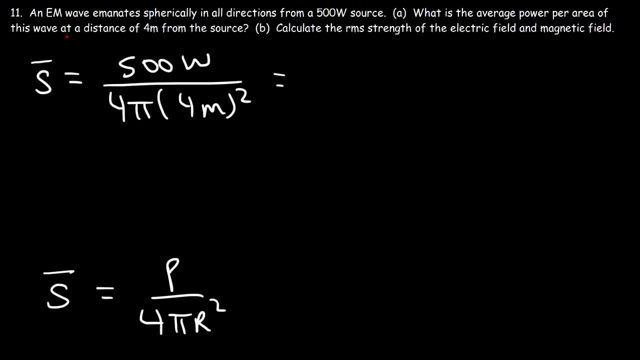 So this is going to be 2.487 watts per square meter. Now calculate the RMS strength of the electric field and the magnetic field using that value. So what formula should we use? Well, we could use this one. So, if we use the RMS electric field, this is going to give us the average S value. 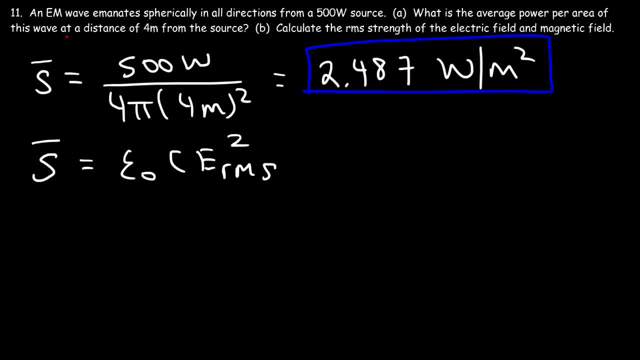 And we don't need the one-half in front of it. We need the one-half if we're using the peak electric field. So let's focus on this formula. So the average S value is 2.487. epsilon sub naught. 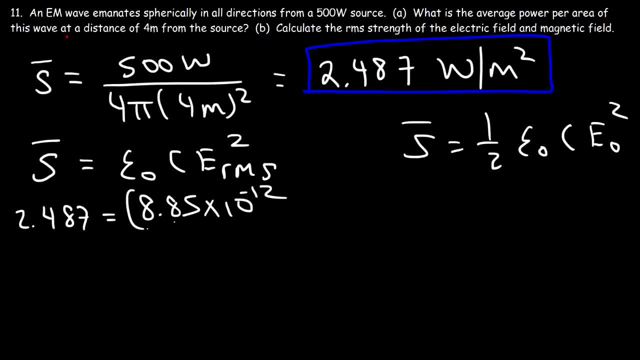 That's 8.85 times 10 to the minus 12.. And the speed of light is 3 times 10 to the 8.. So first let's take 2.487 and divide it by 8.85 times 10 to the minus 12.. 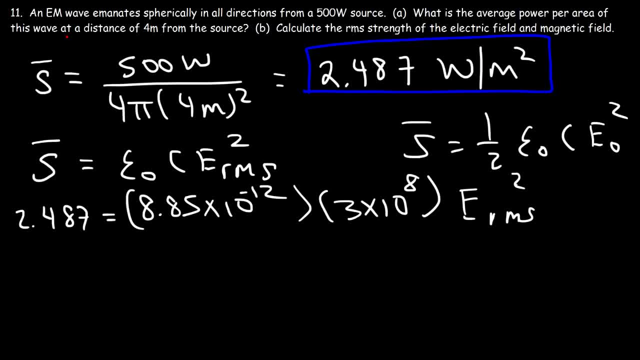 And then take that result and divide it by 3 times 10 to the 8. And then take the square root of your answer. So this will give us The value of the electric field, which is 30.6 newtons per coulomb. 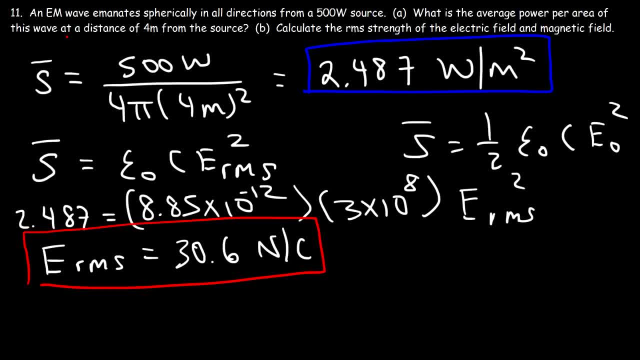 Now let's calculate the RMS strength of the magnetic field. So we're going to use this equation. It's going to be C divided by mu, naught times B RMS squared. So keep in mind, if you have the one-half in front of it, 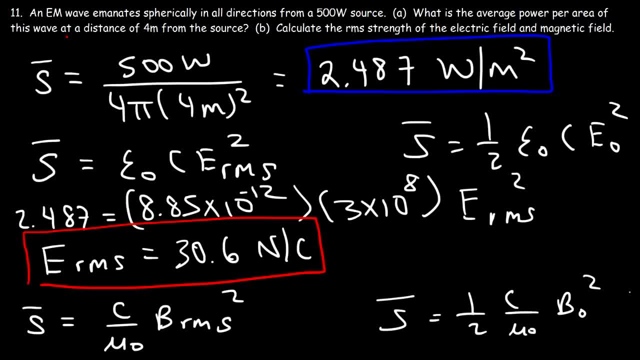 then this would be the peak value of the magnetic field. But if you don't have the one-half just, You can replace that with the RMS value of the magnetic field. So first let's rearrange the equation. I'm going to multiply both sides by mu naught. 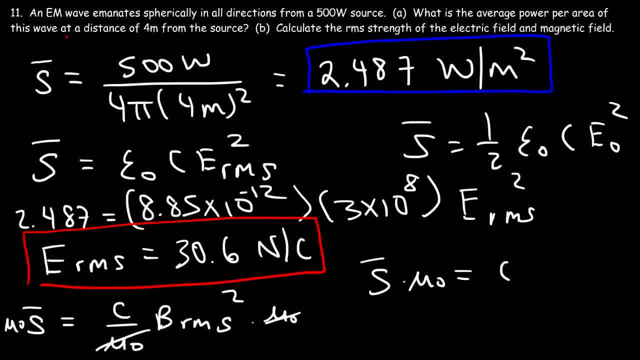 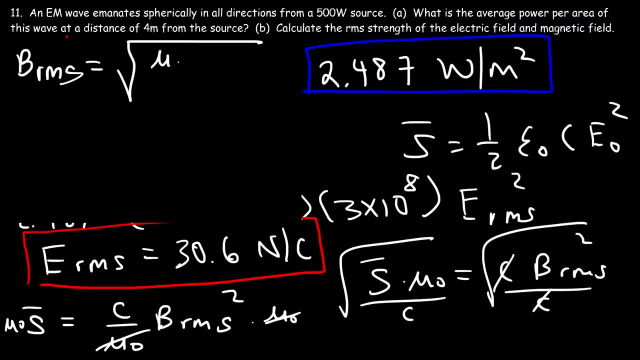 And so we have S times mu naught is equal to C times B RMS. Then I'm going to divide both sides by C And then take the square root. So the RMS strength of the magnetic field is going to be the square root of mu naught times the average S value divided by C. 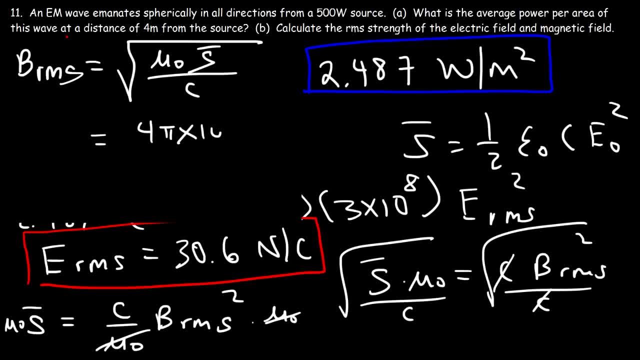 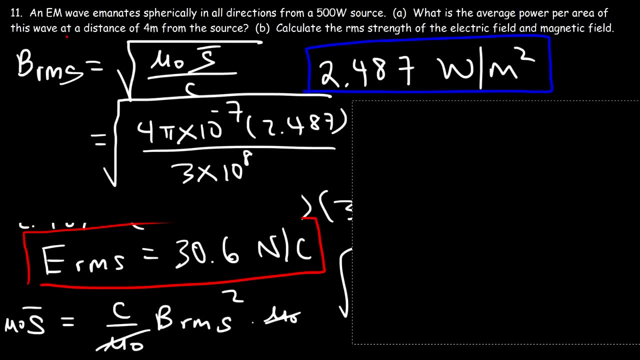 And so mu naught is 4 pi times 10 to the minus 7.. The average S value is 2.487.. And then the speed of light is 3 times 10 to the 8 meters per second. So you should get 1.02 times 10 to the negative 7 Tesla. 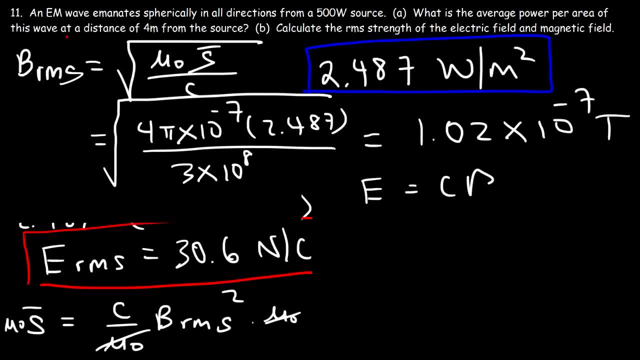 Now keep in mind, the electric field is equal to C times the magnetic field. So if we divide the electric field by the magnetic field, it should give us the speed of light. So if you take 30.6 divided by 1.02 times 10 to the minus 7,,